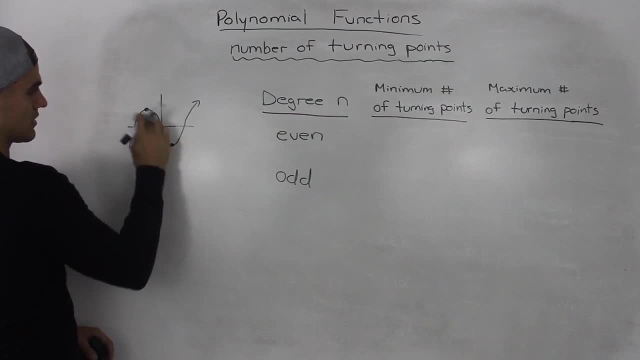 maximum or a minimum. So in this case there are two turning points. a parabola that looks like this, let's say, only has one turning point. A line that looks like this has no turning points. there's no minimum or maximum value. So wherever the function changes shape or hits a maximum or 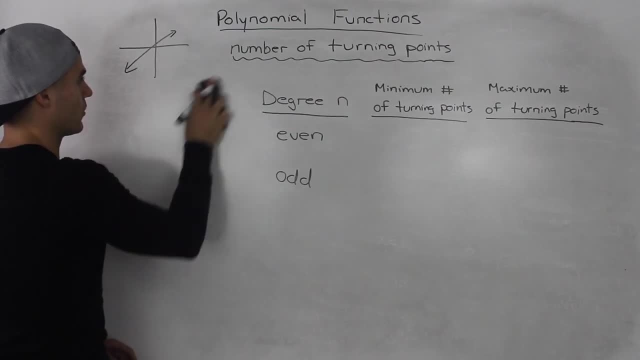 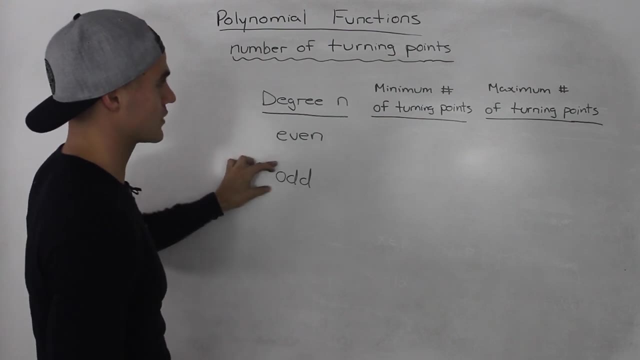 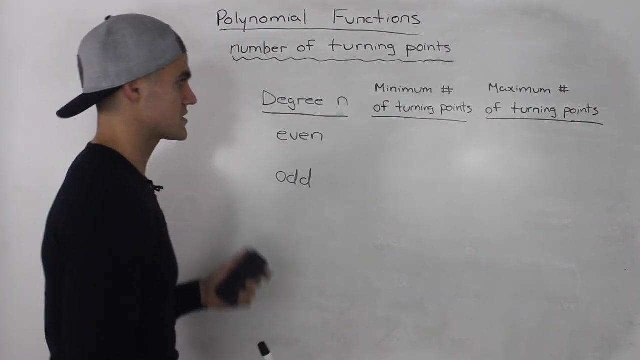 hits a minimum. that's basically what a turning point is. So let's figure out, depending on whether a function has an even degree or an odd degree, what the minimum and maximum number of turning points there are. So let's start off with the maximum number of turning points. It's always equal to whatever. 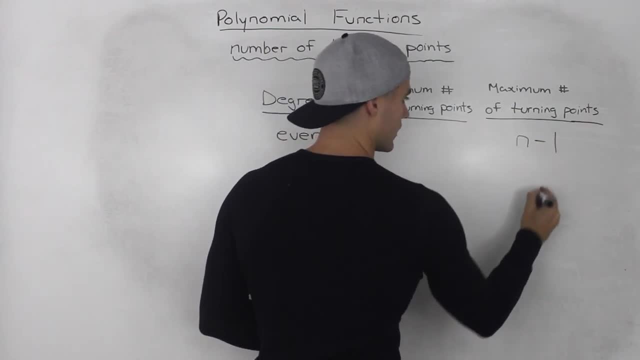 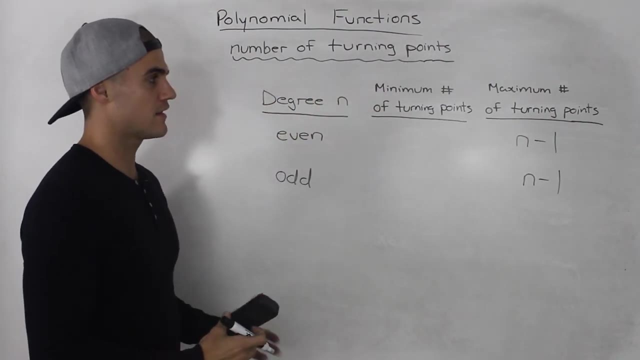 the degree is minus one, and for an odd function as well. So if a function has a degree of five, then there can only be a maximum of four turning points. If it has a degree of three, there can only be two turning points. And a simple example, for that is a parabola. A parabola has a degree. 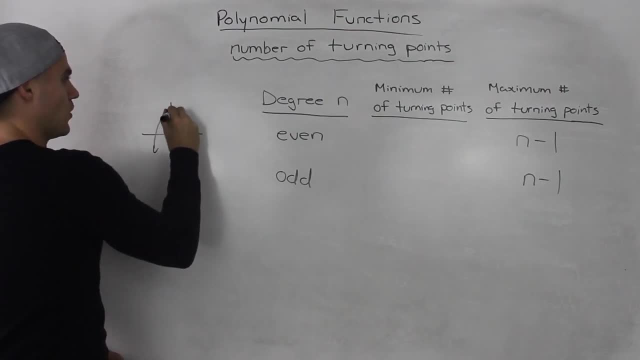 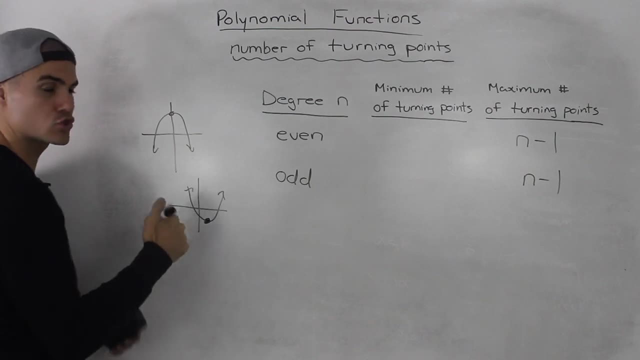 of two and it always No. But as a function, if it has an even degree, then it has an even degree. So what happens is that the function has an even degree, but the degree of four turns points only has one turning point Right. It can either be a maximum or a minimum There. 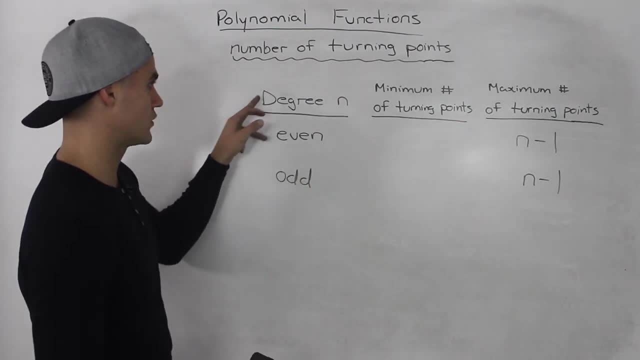 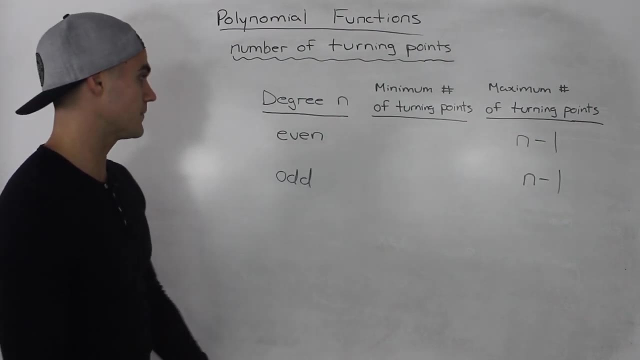 can never be two turning points, So the maximum number of turning points is always equal to n minus one, no matter whether the degree is even or odd. Now let's talk about the minimum number of turning points for a function that has an even degree. And if it has an even degree, 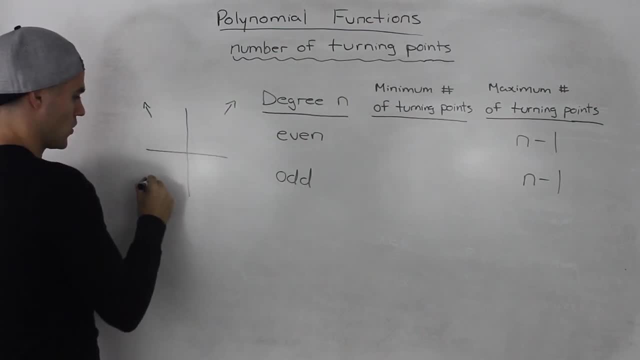 end in quadrant one if it's a positive leading coefficient, or it's going to start in quadrant three and end in quadrant four. so we know that there's going to have to be at least one turning point somewhere, because it could have multiple turning points, but we know that there has to be. 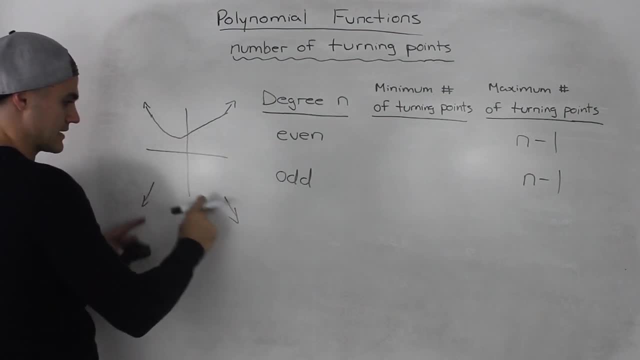 at least one, because it has to come back around. it has the same end behaviors, so this can be have multiple turning points, so one, two and three, but we know that it has to have at least one, whether it's a even degree with a positive leading coefficient or a negative one, because it has to